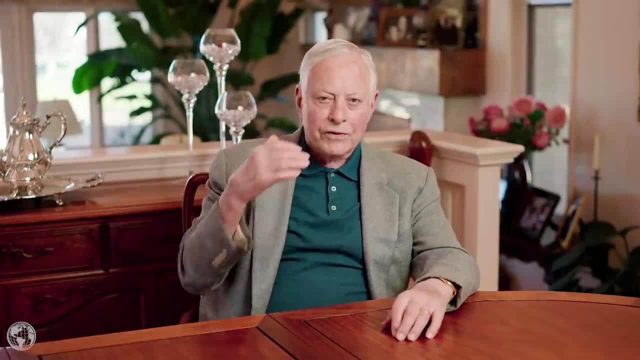 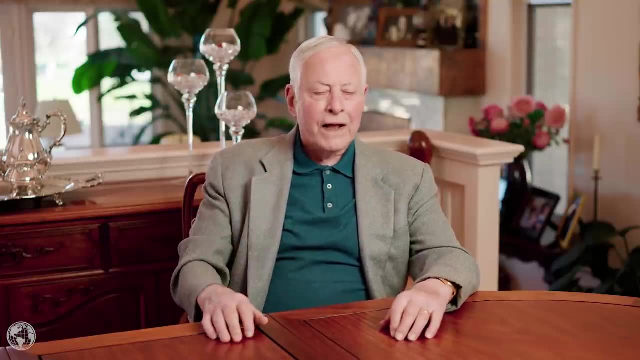 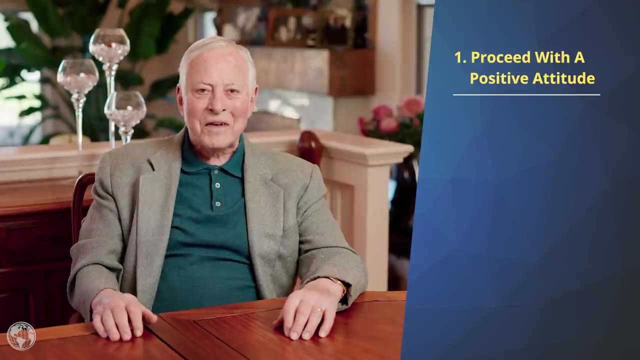 of your thinking, Sort of like a recipe in the kitchen for making a delicious dish. you have a recipe for problem solving that enables you to handle anything that life throws your way. The first step is to proceed with a positive attitude, Approach any problem with the knowledge that there's a practical 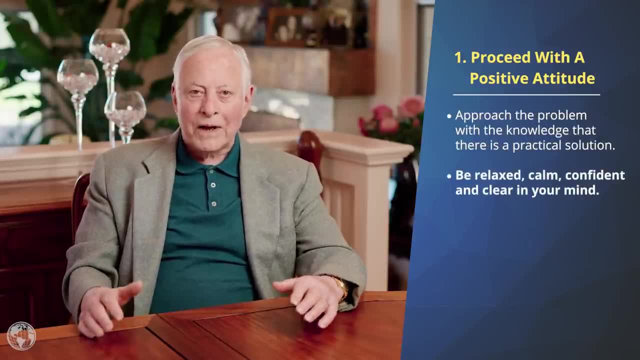 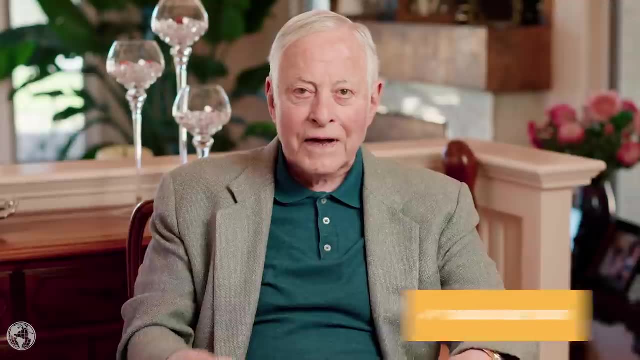 solution just waiting to be found. Be relaxed and calm and confident and clear in your mind. If you're struggling, act as though it were impossible to fail. Act as though you already had a high level of confidence in yourself. If you're struggling, act as though you already had a high 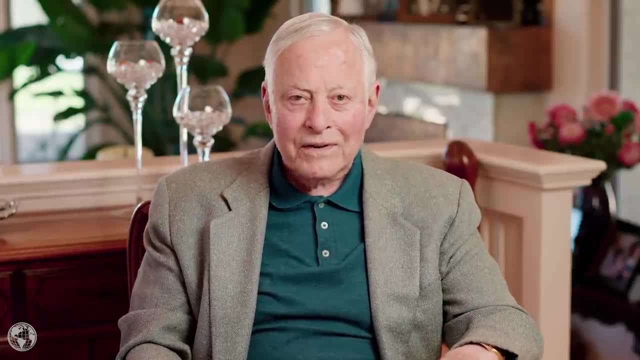 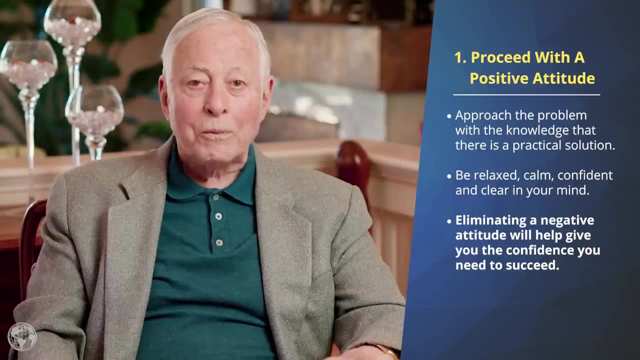 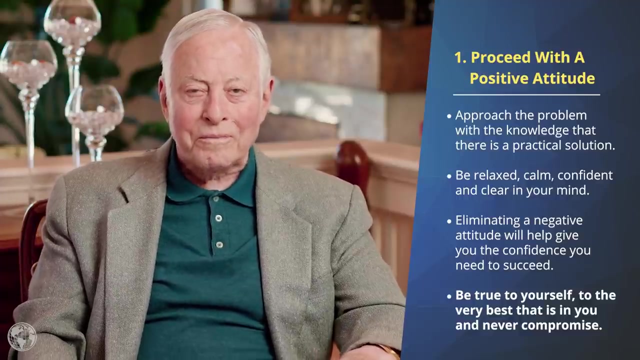 level of self-confidence and that success was guaranteed. Eliminating a negative attitude about the outcome of your goal will help give you the confidence that you need to succeed. Be true to yourself, to the very best that is in you, and never compromise. The next step is to define the 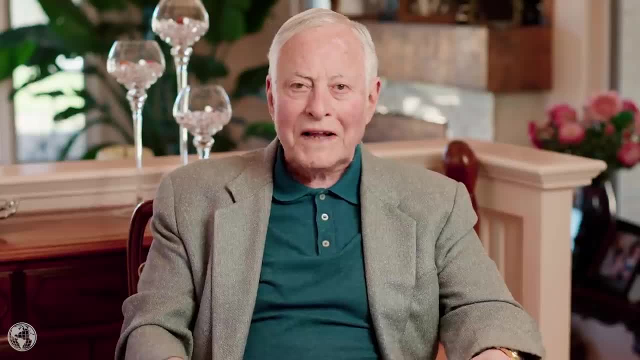 problem clearly. Define the problem clearly in writing. It's absolutely astonishing when I work with a group of examiners who have a very high level of self-confidence and that success was guaranteed. Eliminating a negative attitude about the outcome of your goal will help give you the 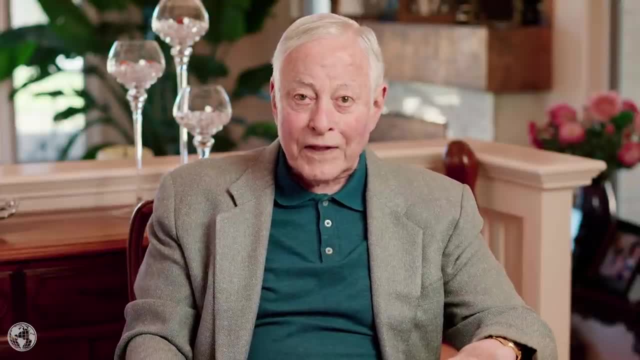 confidence that you need to succeed. Be true to yourself, to the very best that is in you, and never compromise. The next step is to write down a definition that they're working with in the company. Every person will have a different definition of the same problem, which is why 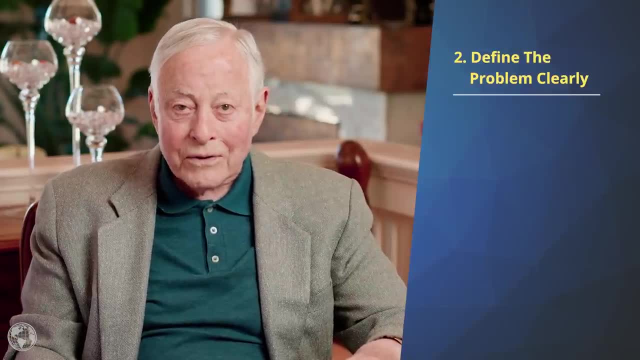 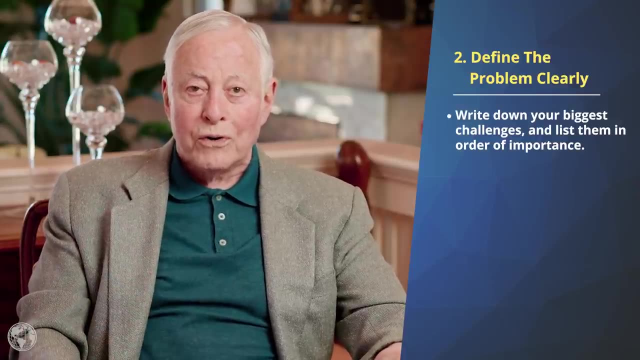 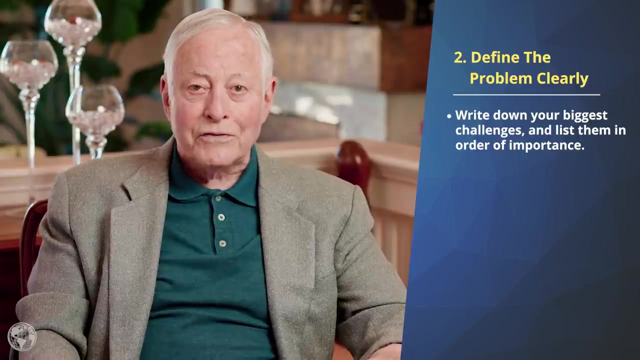 they never get it solved. The first thing you do every morning should be to write down your biggest challenges, the obstacles that stand between you and your goal, and then list them in order of importance. If you do this one simple step, you'll immediately see your productivity. 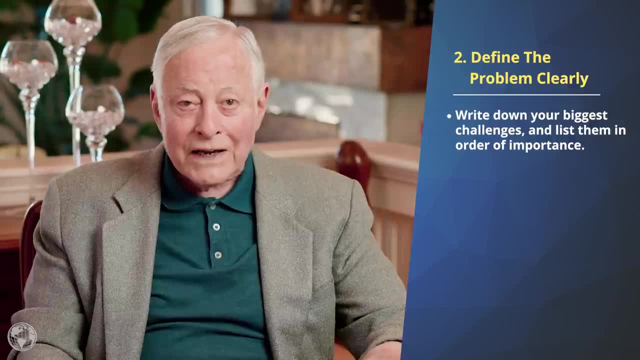 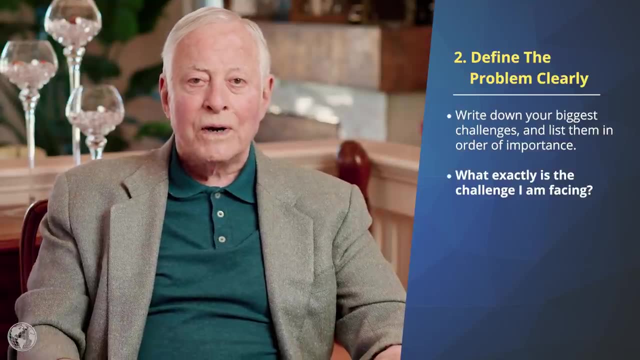 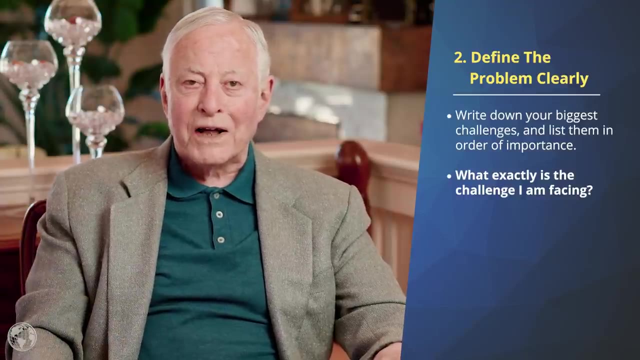 performance and your self-confidence increase by 25% or more. If you're not sure where to start, try asking what exactly is the challenge that I'm facing. Never use problem. The very best word is always a challenge or obstacle. 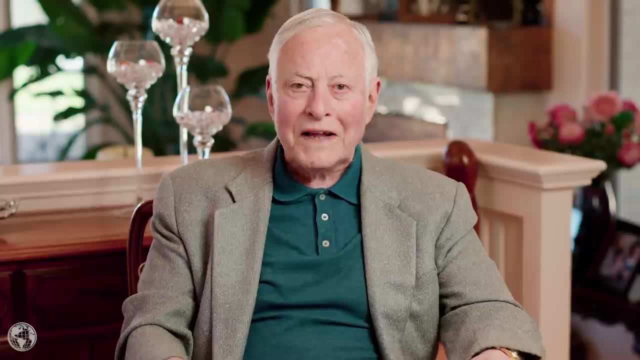 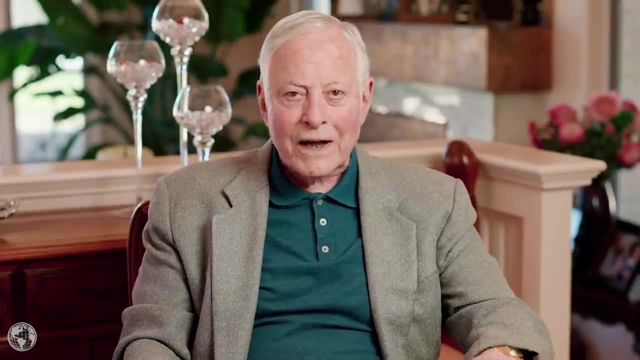 problem clearly. Define the problem clearly in writing. It's absolutely astonishing when I work with a group of executives who have a very high level of self-confidence and that success was guaranteed. I'll have each person write down a definition that they're working with in the 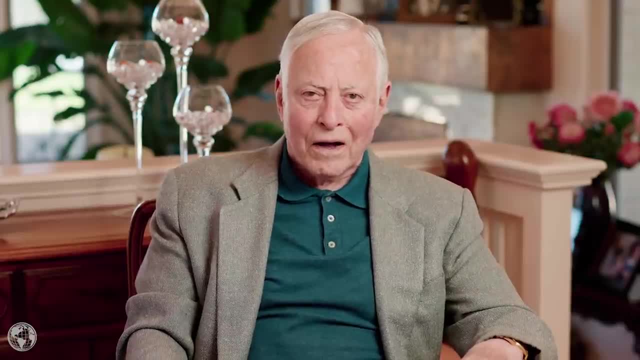 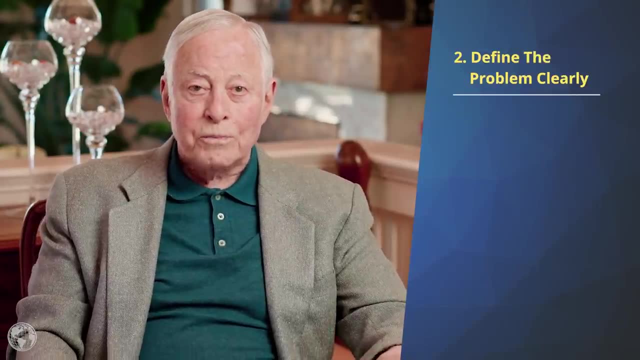 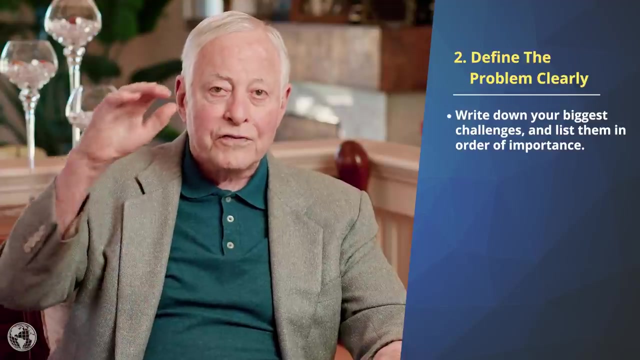 company and everyone will have a different definition of the same problem, which is why they never get it solved. The first thing you do every morning should be to write down your biggest challenges, the obstacles that stand between you and your goal, and then list them. 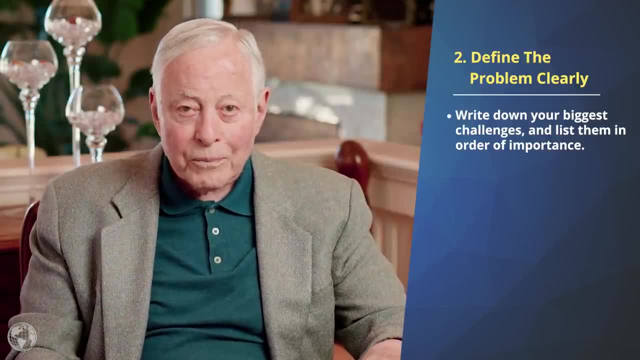 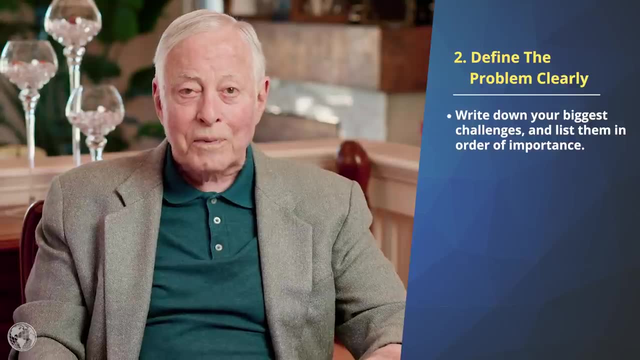 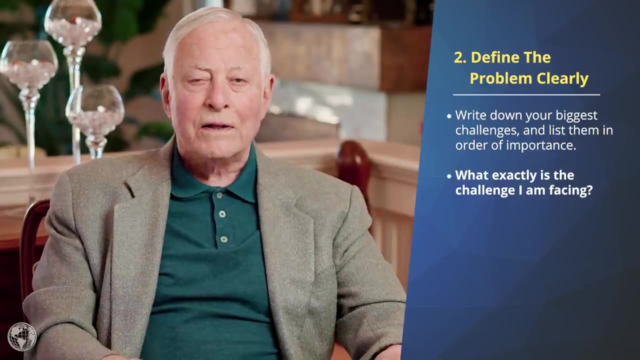 in order of importance. If you do this one simple step, you'll immediately see your productivity performance and your self-confidence increase by 25% or more. If you're not sure where to start, try asking what exactly is the challenge that I'm facing. Never use problem, The very best word. 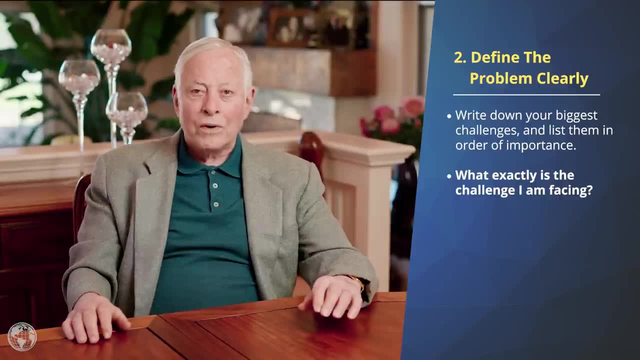 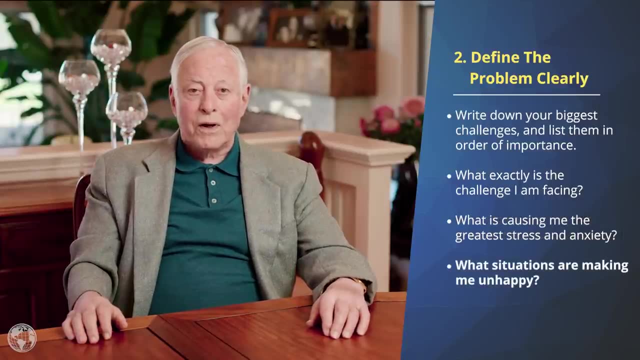 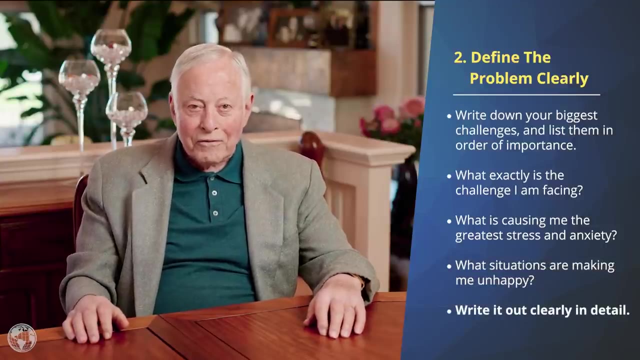 is always a challenge or obstacle. What is causing me the greatest stress and anxiety in my life right now? What situations or problems are making me unhappy or doubtful? Write it out clearly in detail. Fully 50% of situations can be resolved by accurate. 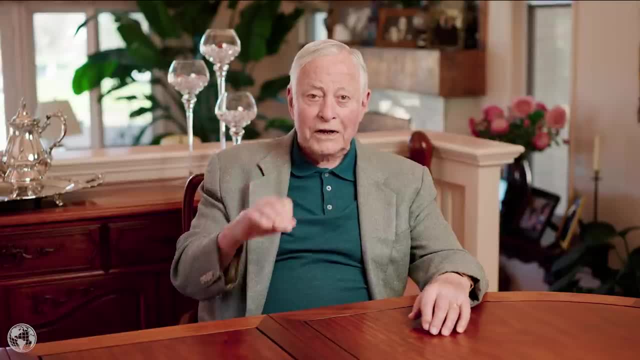 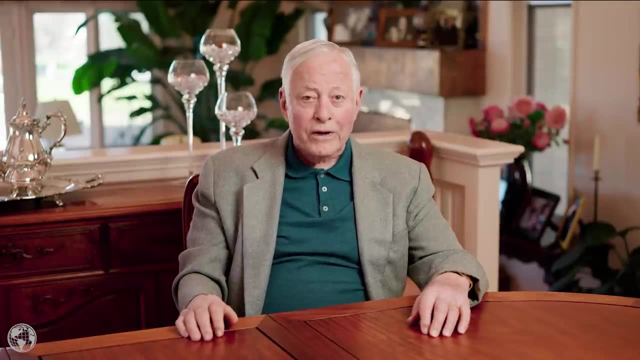 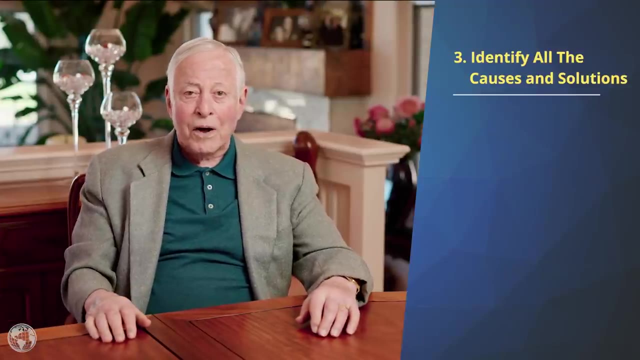 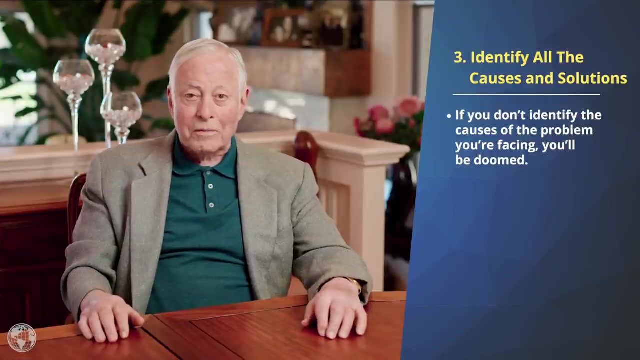 definition. Just by clearly defining your problems and your goals and looking at ways to make progress, you'll be well on the way to tackling anything that comes your way. Next, identify all the causes and possible solutions to the problems you are facing. If you don't identify the causes of the problem you're facing, you'll be doomed like Sisyphus. 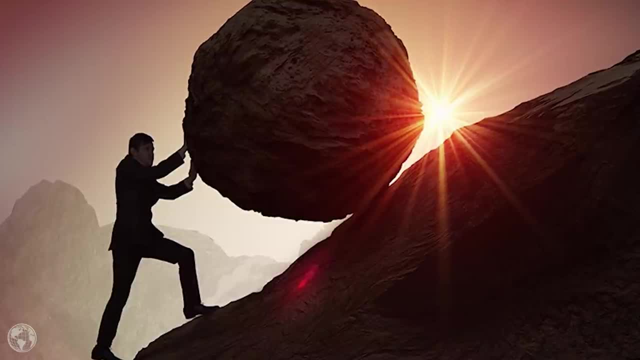 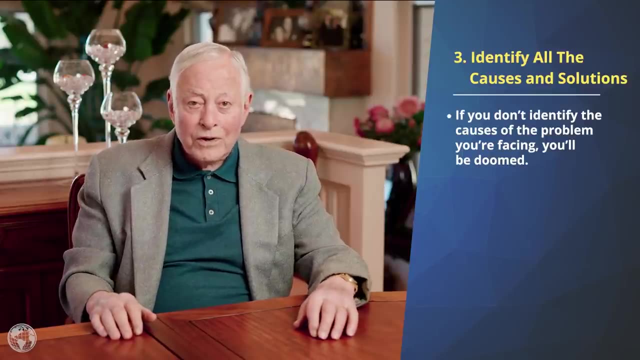 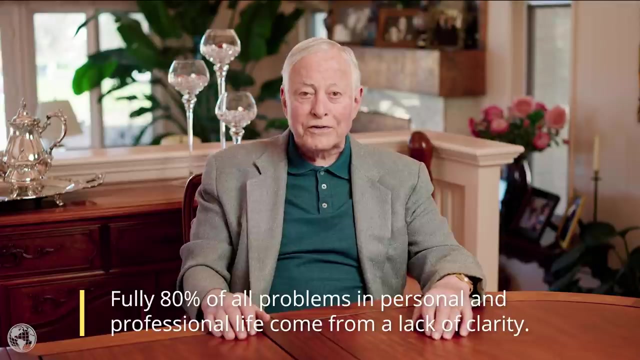 pushing the boulder up the hill and the boulder keeps rolling back down again, to deal with the same issues again and again. That's why you need to search for the root cause of the problem. Fully 80% of all problems in personal and professional life come from a lack of clarity. What exactly? 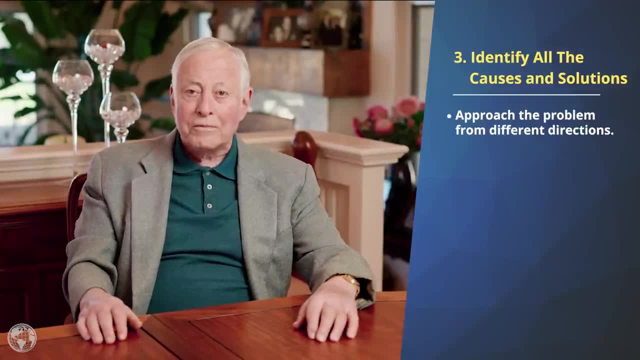 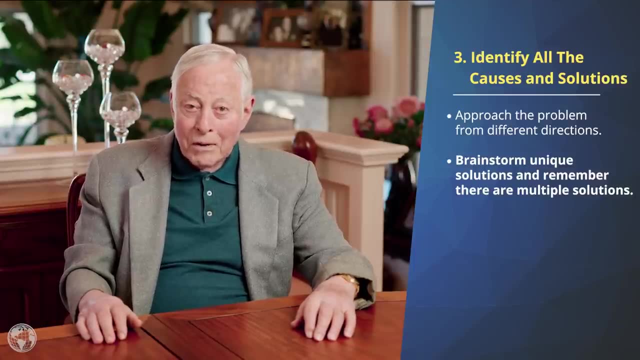 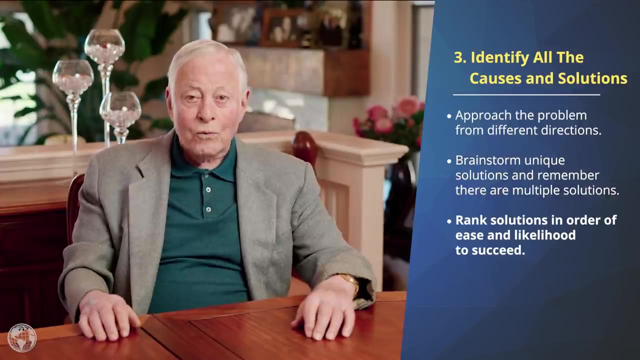 is the problem. Approach the problem from different directions, Brainstorm unique solutions And remember there are likely multiple solutions to the same problem, not just one. Once you've written your solutions down, rank them in order of ease and likelihood to succeed. Then start. 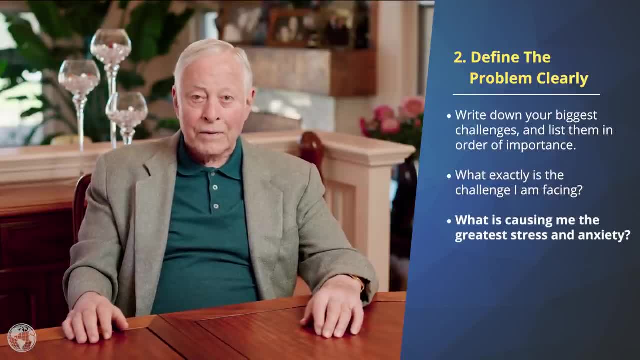 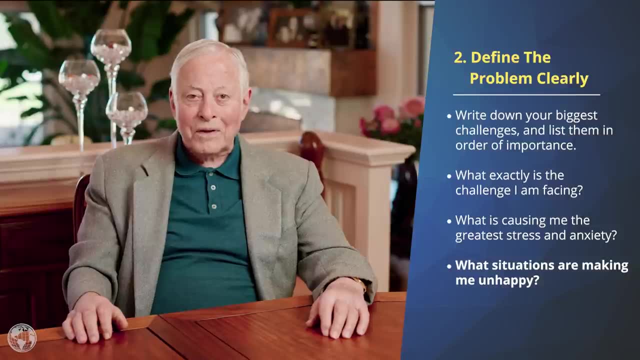 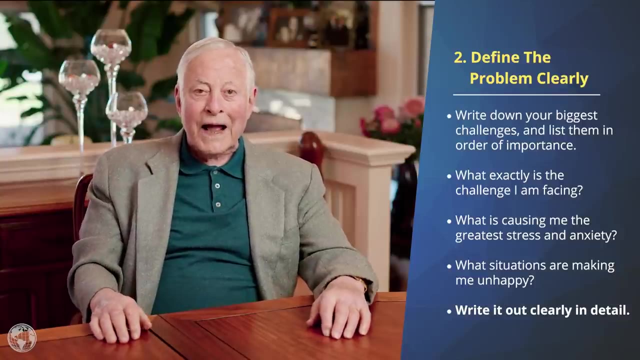 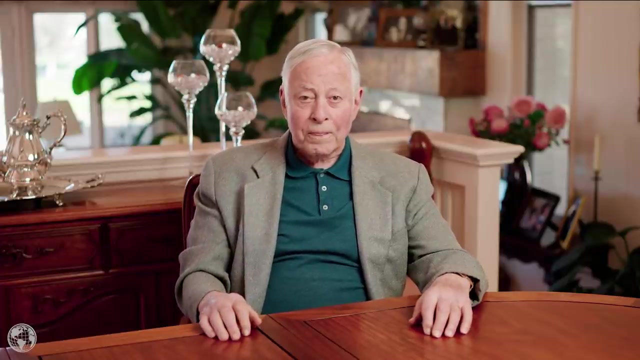 What is causing me the greatest stress and anxiety in my life right now? What situations or problems are making me unhappy or doubtful? Write it out clearly in detail. Fully 50% of situations can be resolved by accurate definition, Just by clearly defining your problems and your goals and looking at ways to make progress. 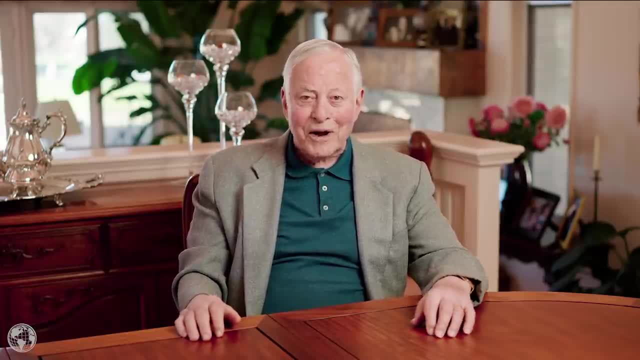 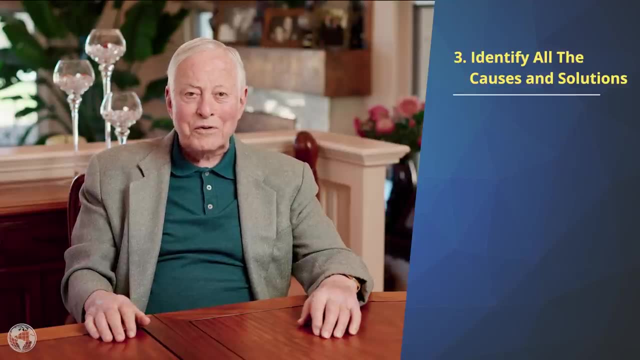 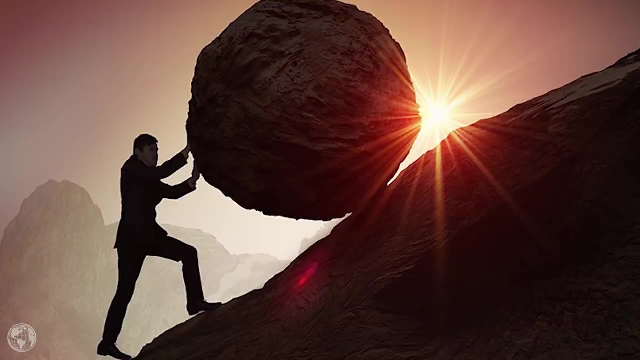 you'll be well on the way to tackling anything that comes your way. Next, identify all the causes and possible solutions to the problems you are facing. If you don't identify the causes of the problem you're facing, you'll be doomed like Sisyphus. 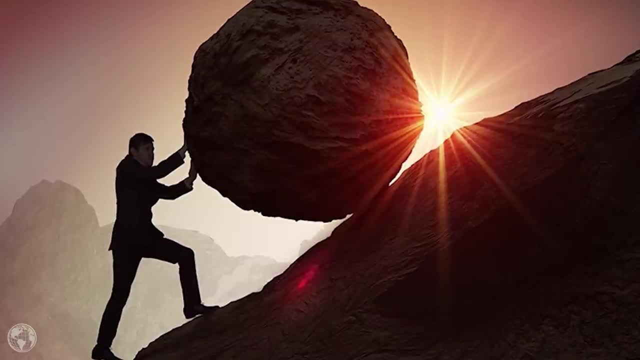 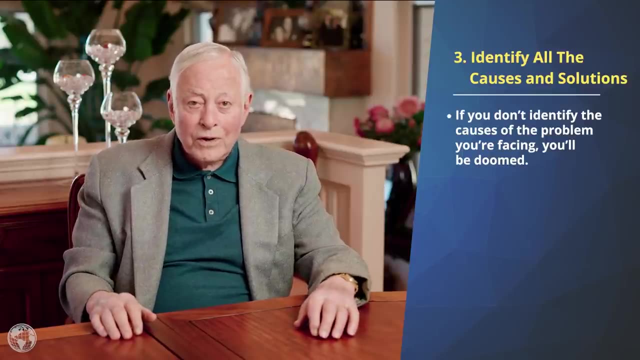 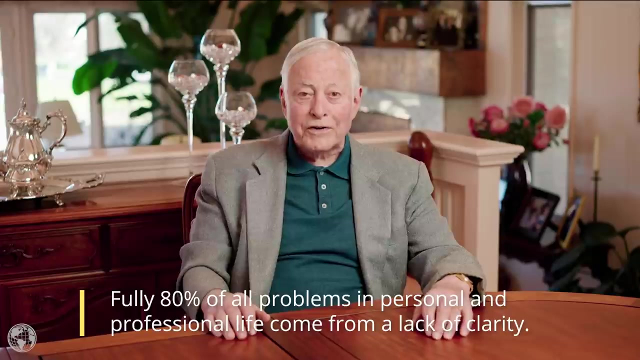 pushing the boulder up the hill and the boulder keeps rolling back down again, to deal with the same issues again and again. That's why you need to search for the root cause of the problem. Fully 80% of all problems in personal and professional life come from a lack of quality. 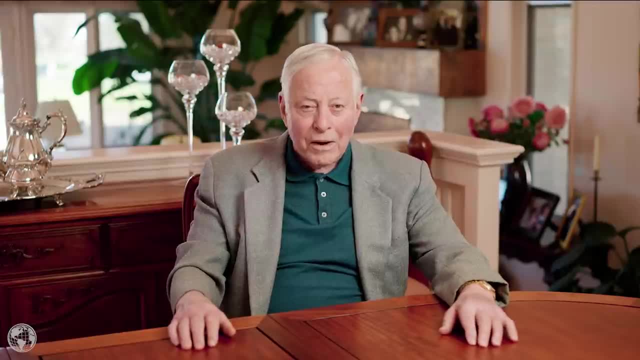 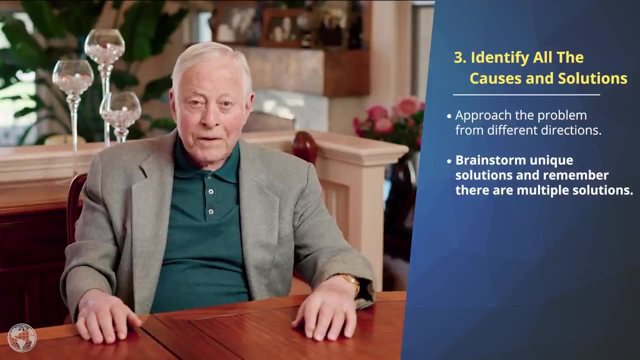 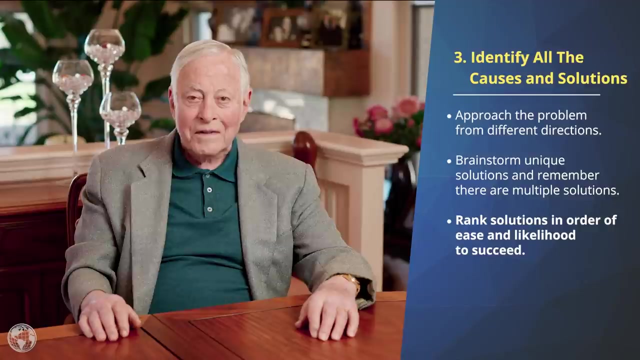 What exactly is the problem? Approach the problem from different directions, Brainstorm unique solutions And remember there are likely multiple solutions to the same problem, not just one. Once you've written your solutions down, rank them in order of ease and likelihood to succeed. 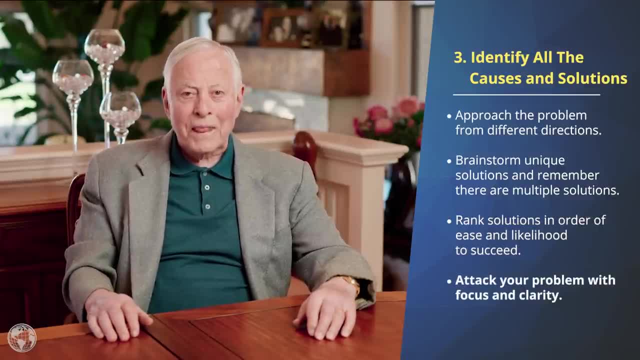 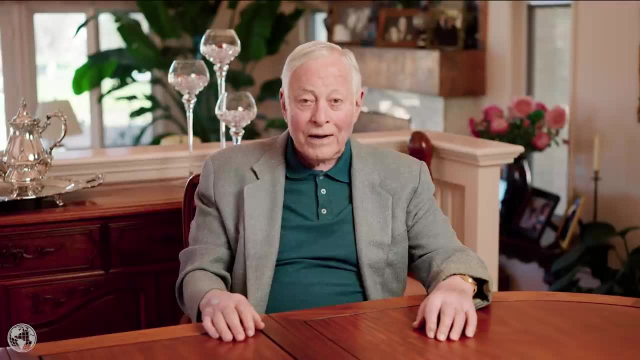 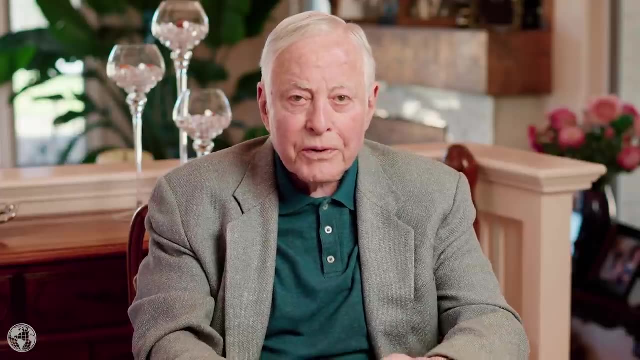 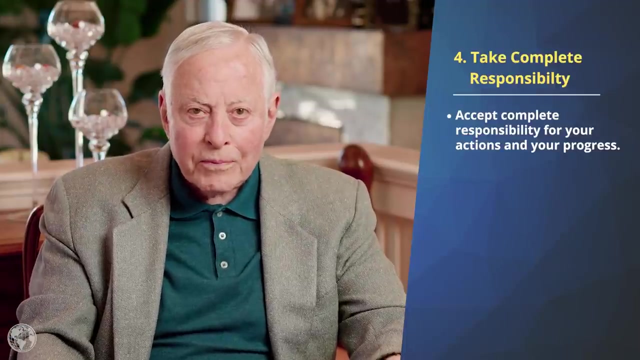 Then start attacking your problem with focus and clarity. And don't worry if your first solution doesn't work. you'll be ready to try the next tactic on your list. The fourth step is for you to take complete responsibility for your decisions. Remember, if it's to be, it's up to me. 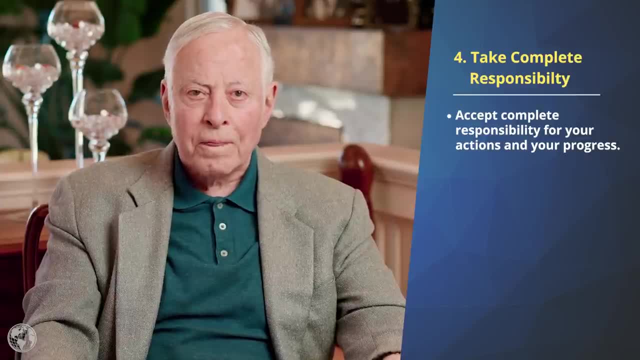 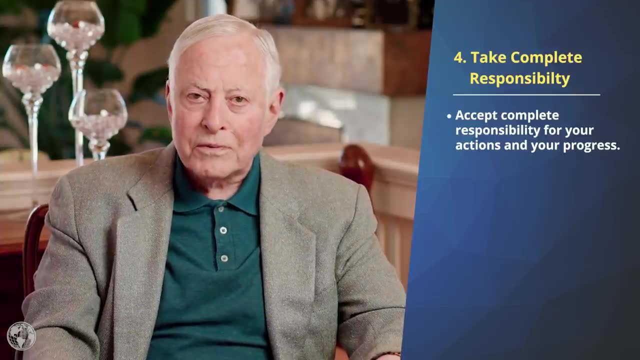 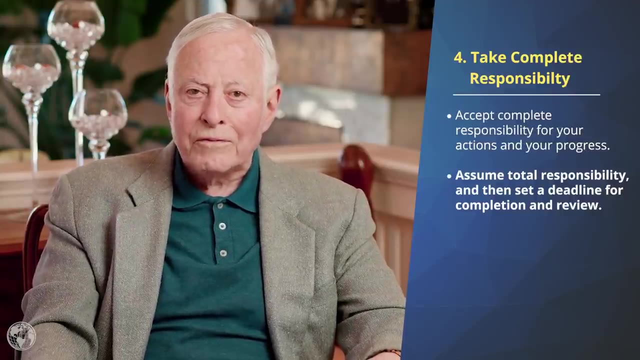 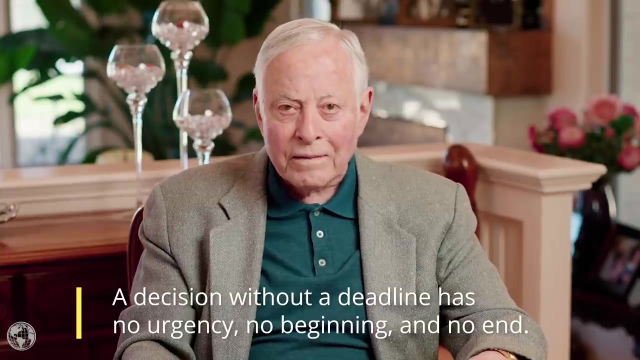 Accept complete responsibility for your actions and your progress. Many of the most creative ideas never materialize because no one accepts responsibility. So let's start Assume total responsibility and then set a deadline for completion and review. Remember, a decision without a deadline has no urgency, no beginning and no end. 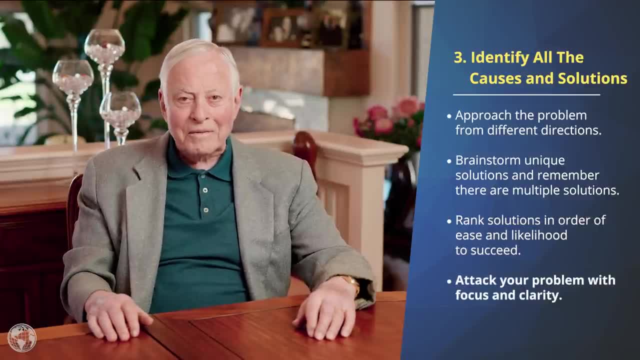 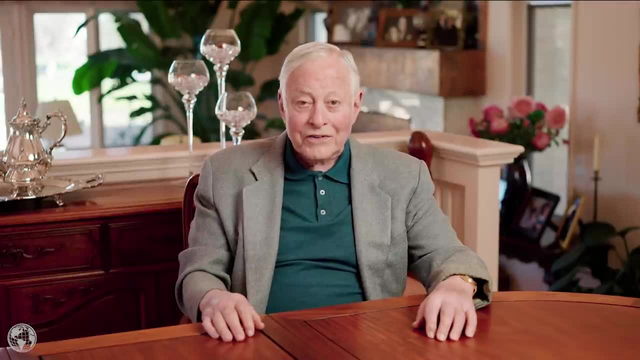 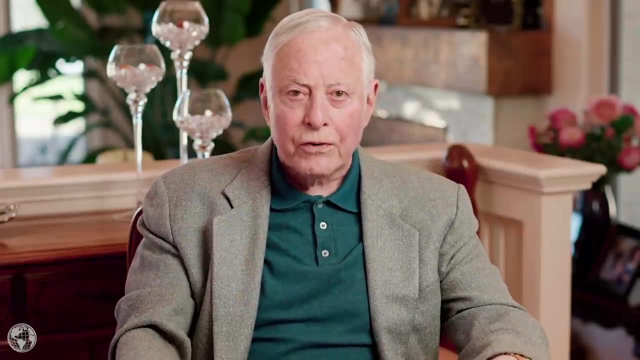 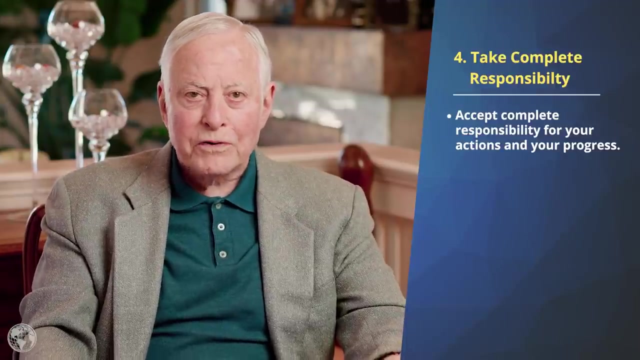 attacking your problem with focus and clarity. And don't worry, if your first solution doesn't work, You'll be ready to try the next tactic on your list. The fourth step is for you to take complete responsibility for your decisions. Remember, if it's to be, it's up to me. Accept complete responsibility for your actions and your progress. 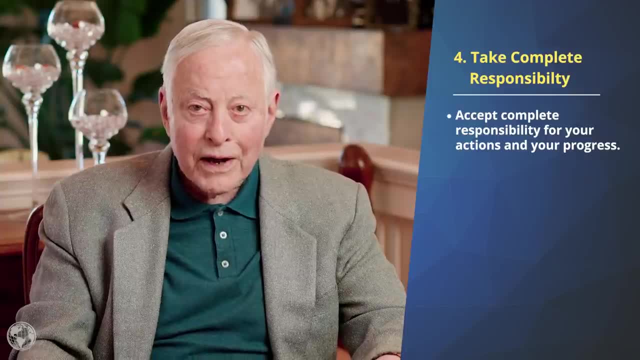 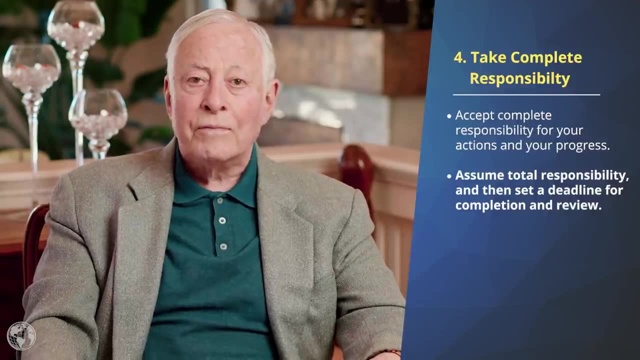 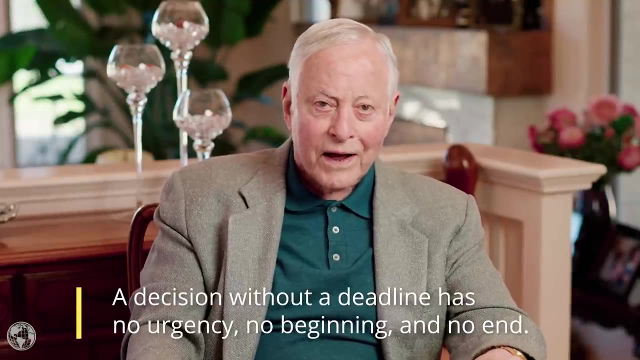 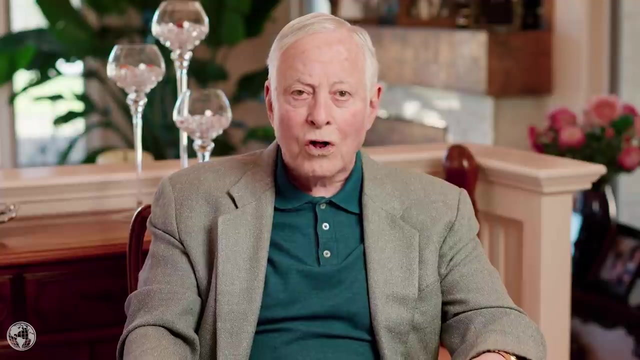 Many of the most creative ideas never materialize because no one accepts responsibility. Assume total responsibility and then take full responsibility. Set a deadline for completion and review. Remember: a decision without a deadline has no urgency, no beginning and no end. The most successful leaders always hold themselves. 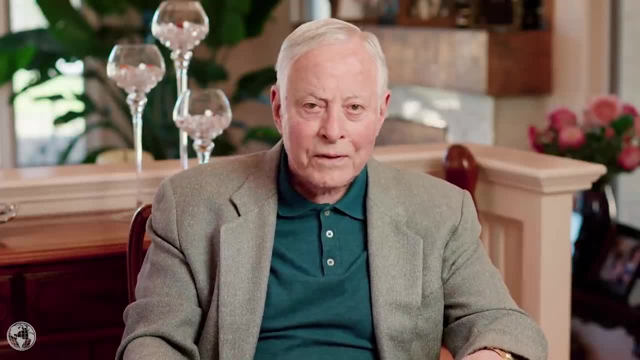 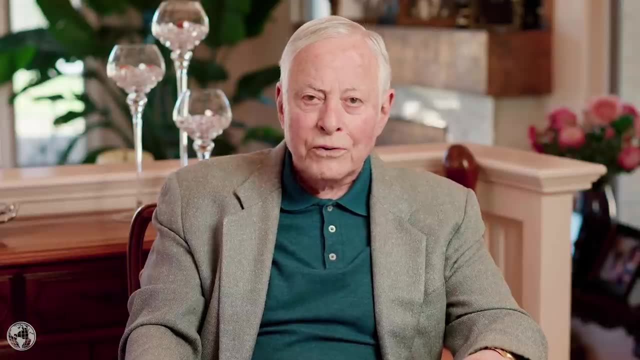 accountable to decisions and deadlines. To become someone that you have never been before, you must take full ownership of your life and do something that you've never done before. Make sure to find the right person to take full responsibility for your actions and your decisions. 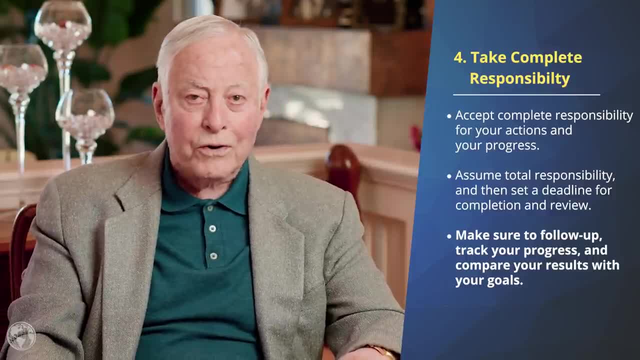 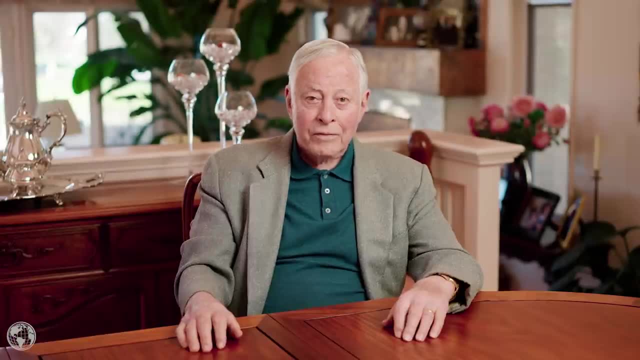 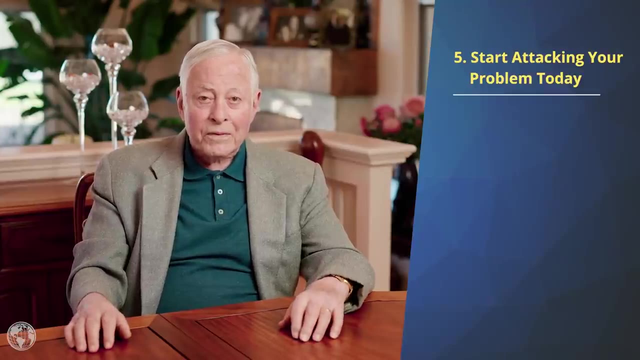 The last step is for you to follow up, Track your progress and compare your results with your goals. The final step is for you to start attacking your problem today. There's never been a better time to start today, not tomorrow and certainly not someday. In order to succeed, you must 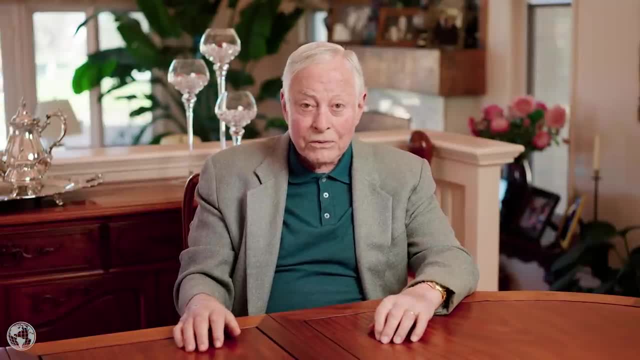 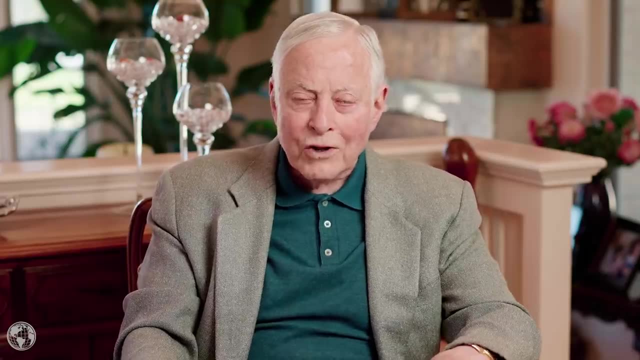 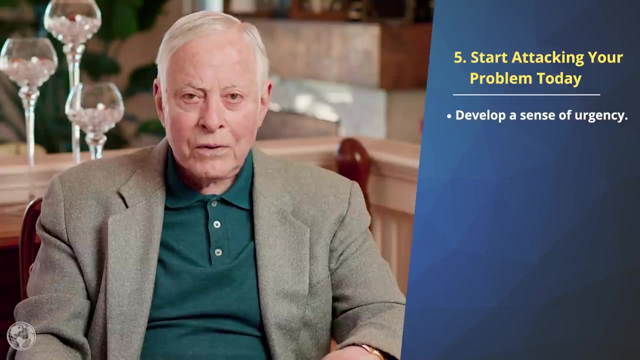 develop a sense of urgency. The faster you move in the direction of your clearly defined goals, the more successful you will be, The more money you will earn and the more you will learn and grow. Remember, you can solve any problem, overcome any obstacle or achieve any goal that you can set for yourself. 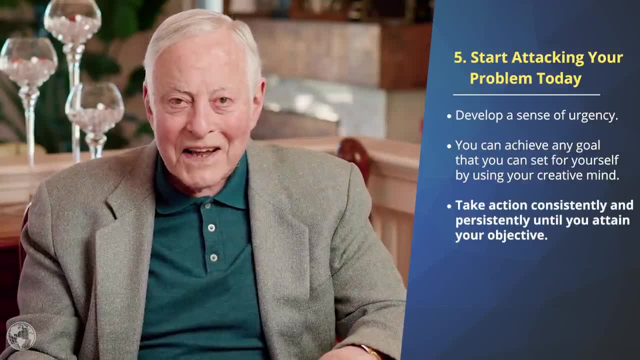 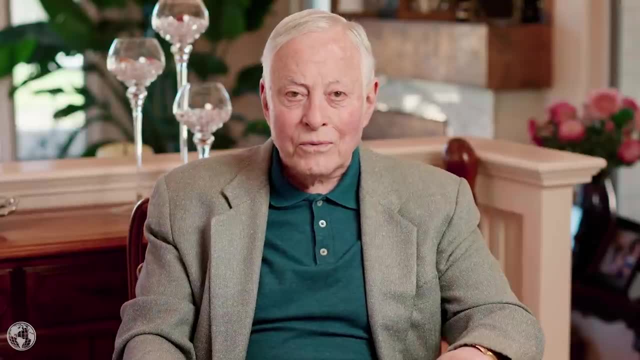 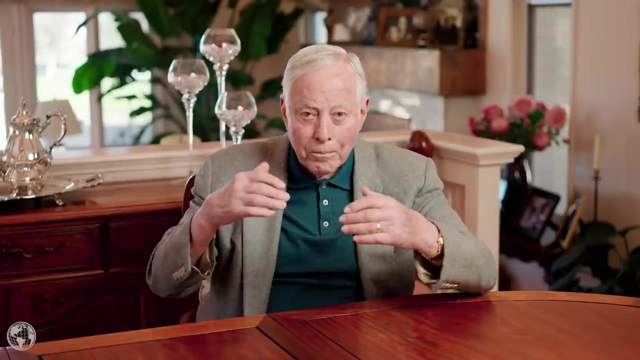 by using your wonderful creative mind and taking action consistently and persistently until you attain your objective. And there are two ways to deal with any setbacks along the way: To carry your problems as bold orders that burden you along the way, or to use your setbacks as stepping stones to 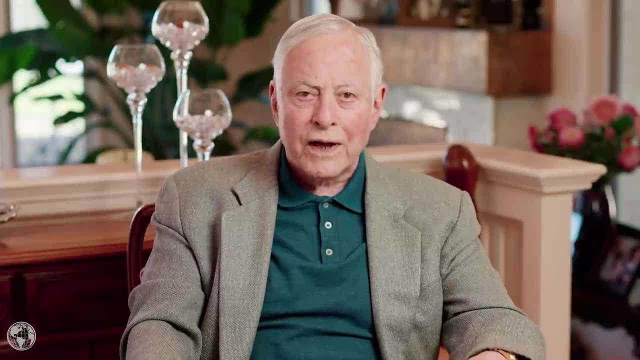 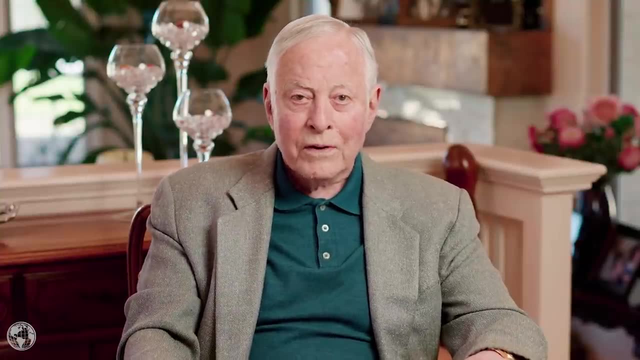 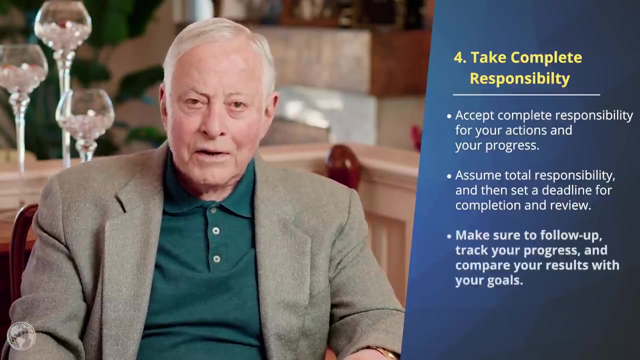 The most successful leaders always hold themselves accountable to decisions and deadlines. To become someone that you have never been before, you must take full ownership of your life. You must do something that you've never done before. Make sure to follow up, track your progress and compare your results with your goals. 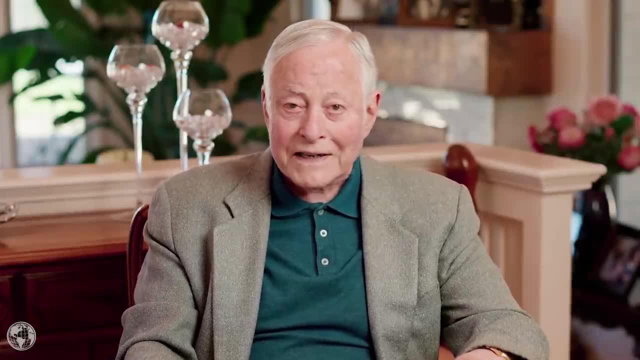 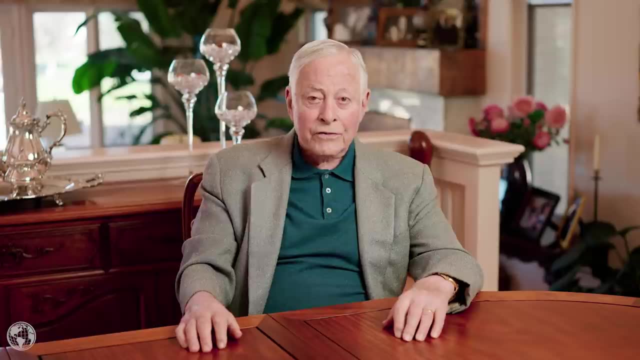 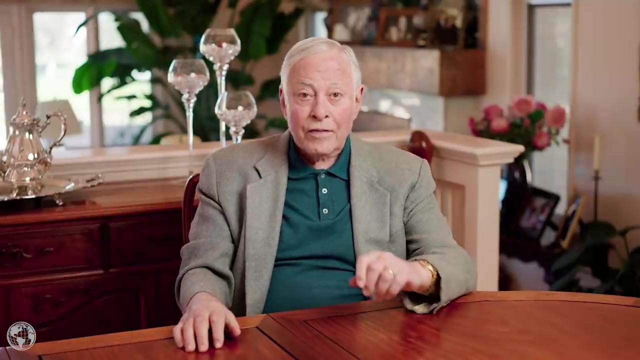 The final step is for you to start attacking your problem today. There's never been a better time to start today, Not tomorrow and certainly not someday. In order to succeed, you must develop a sense of urgency. The faster you move in the direction of your goal, the faster you will succeed. 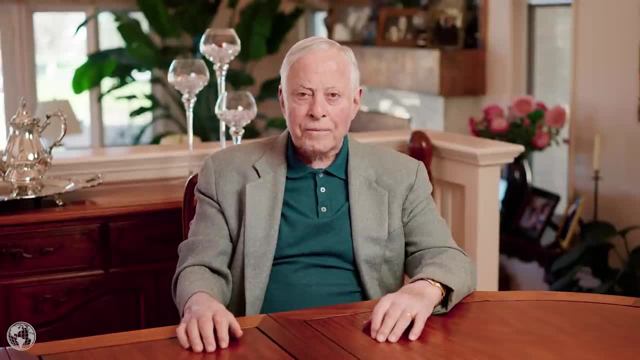 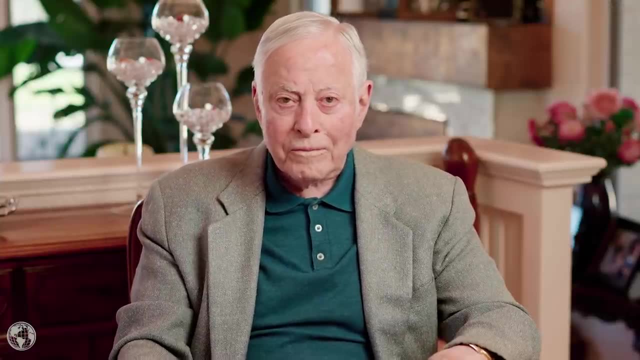 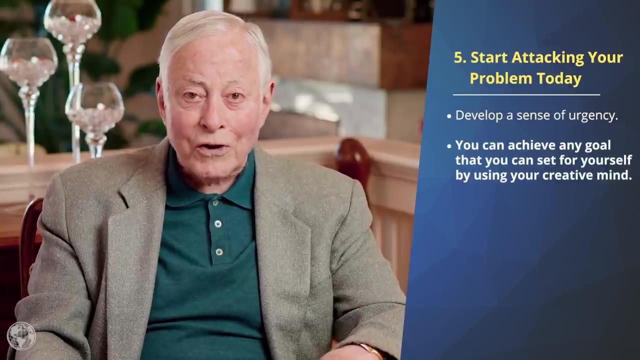 Be the one to be direction of your clearly defined goals. the more successful you will be, the more money you will earn and the more you will learn and grow. Remember, you can solve any problem, overcome any obstacle or achieve any goal that you can set for yourself by using your wonderful creative mind. 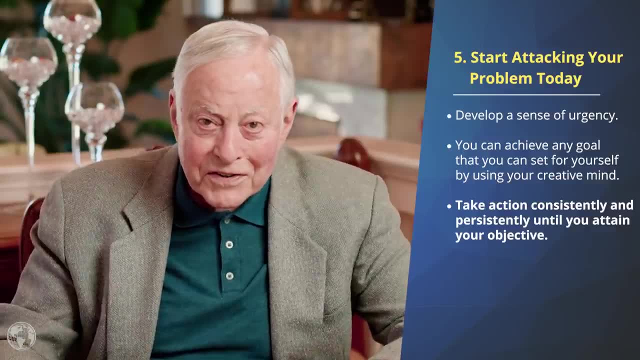 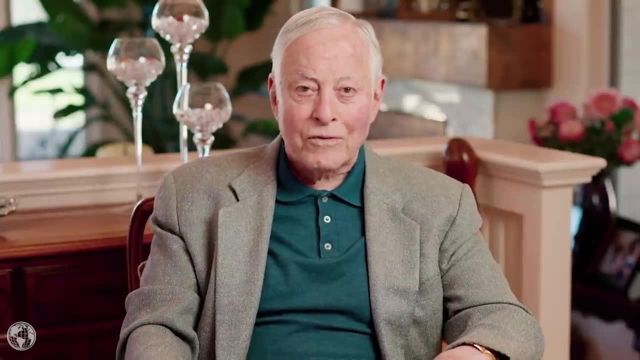 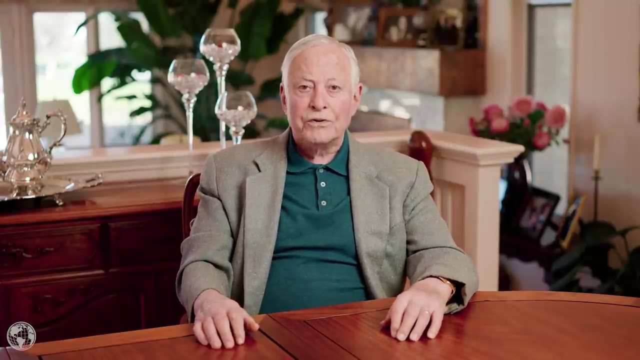 and taking action consistently and persistently until you attain your objective. And there are two ways to deal with any setbacks along the way: To carry your problems as boulders that burden you along the way, or to use your setbacks as stepping stones to pave a new path for yourself. 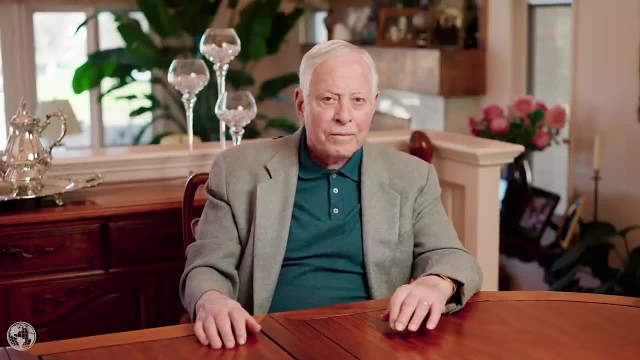 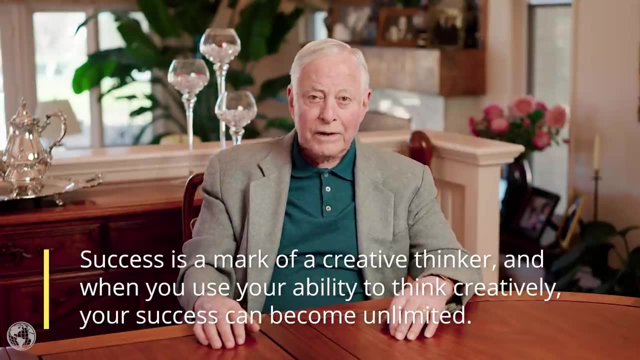 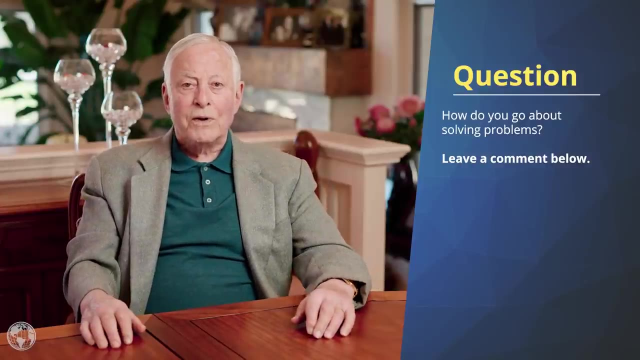 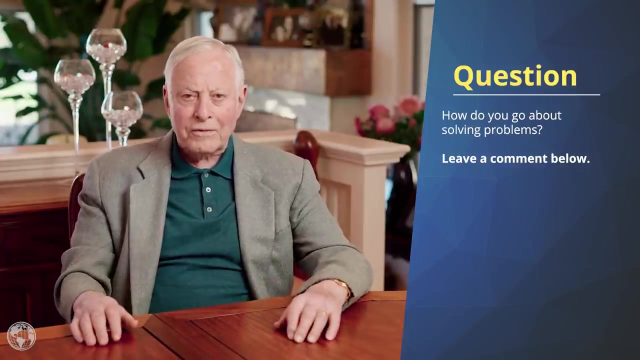 you'll get better and better and stronger and stronger. Success is the mark of a creative thinker, and when you use your ability to think creatively, your success can become unlimited. Now I'd love to hear from you, So my question today is: how do you go about solving problems? What is your method or process? 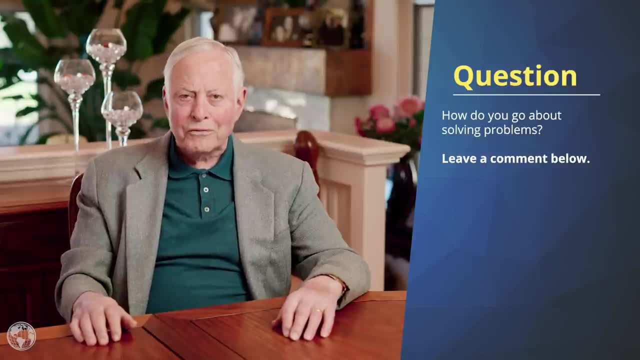 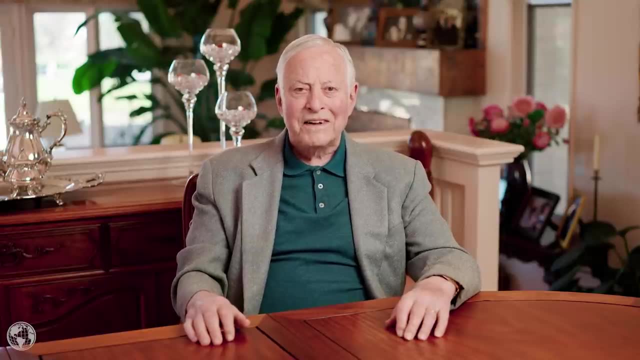 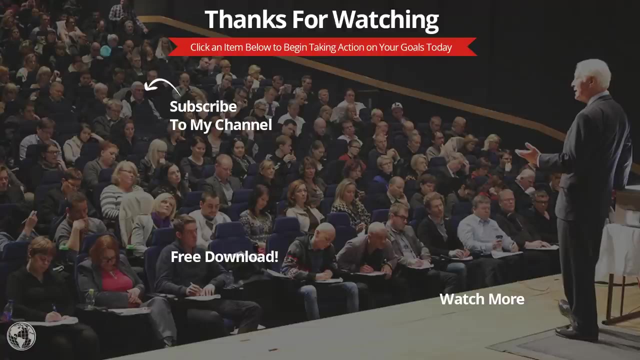 Leave a comment below and I'll be sure to follow up with you. Thanks for watching and remember: if you want to change your future, take action, and take action now, If you enjoyed this video and feel it was valuable in teaching you about the five steps that help you to solve any problem. 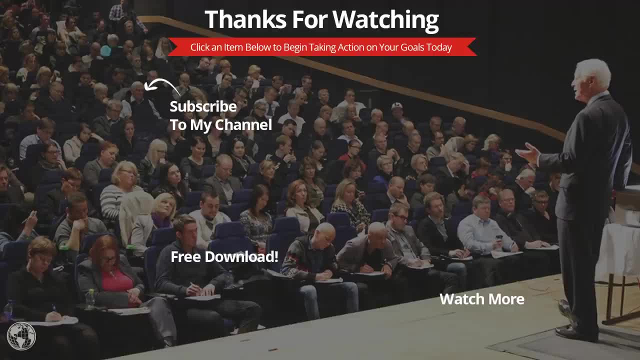 subscribe to my channel and I'll see you in the next video. Like this video and share this video with your friends. Don't forget to click the button on the screen for a free gift. Thanks again for watching.